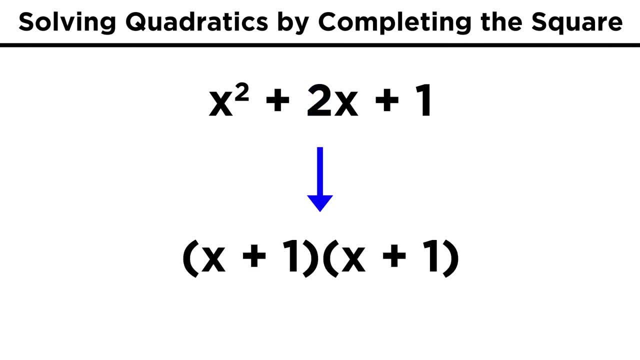 do indeed add up to two, so we can factor this into x plus one. times x plus one- Anything times itself, is by definition that thing squared, so we can also express this as x plus one quantity squared. If this were equal to zero, the solution is very simple. it's just negative one, because 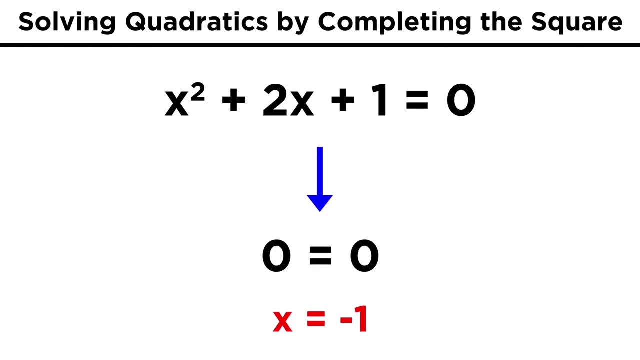 that's the value for x that will make this equal to zero. So the original polynomial must be a perfect square, since it can be generated by squaring this binomial, just like how, four is a perfect square because it's two squared. This kind of thinking comes in handy for certain polynomials. 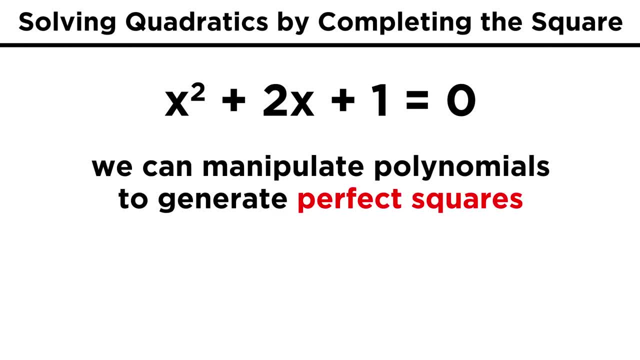 Because, while they might not factor, we can deliberately add some term to the expression. that will manufacture a polynomial that is a perfect square, thus allowing us to express it as the square of a binomial and making it easy to solve. This will make more sense with an example. 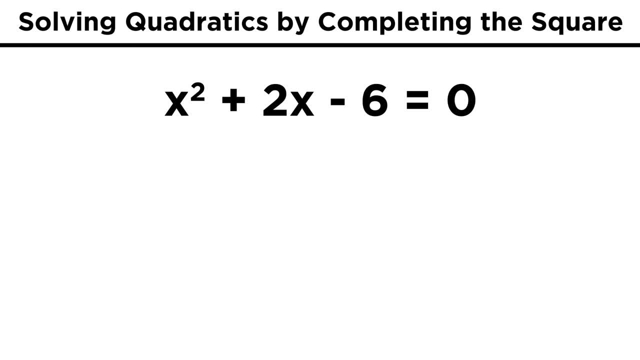 Let's say we have x squared plus two. x minus six equals zero. If we find the factors of negative six, which are combinations of one and six or two and two and three, we find that there is no way to add any pair of factors together to get. 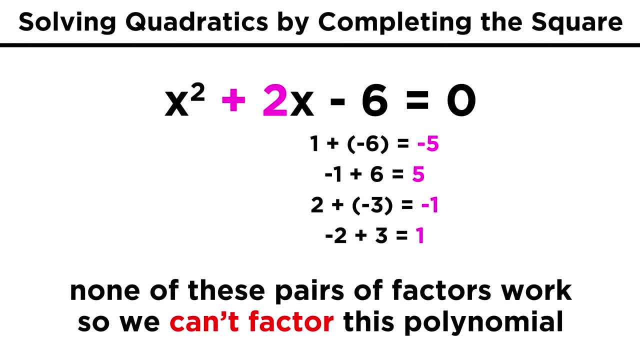 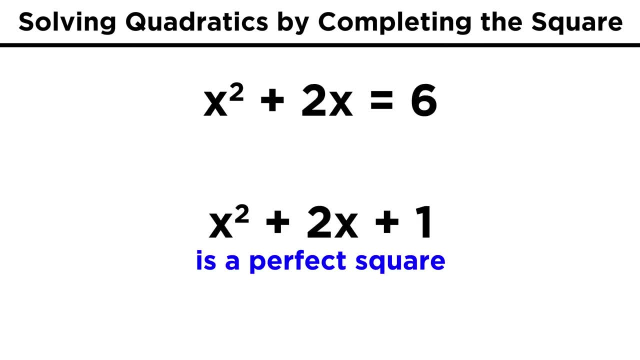 positive two. so we can't factor this polynomial. But let's do a little trick. Let's add six to both sides, bringing the six to the other side. Earlier we saw that x squared plus two, x plus one is a perfect square. so what if we now 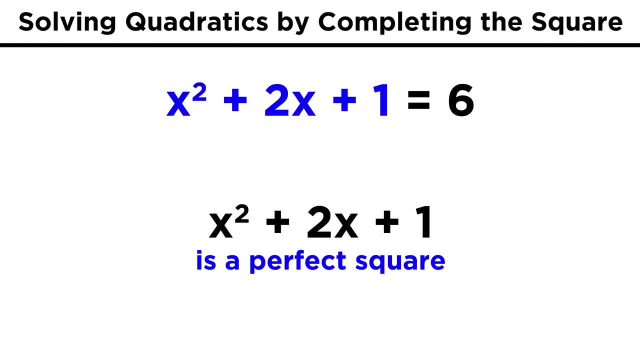 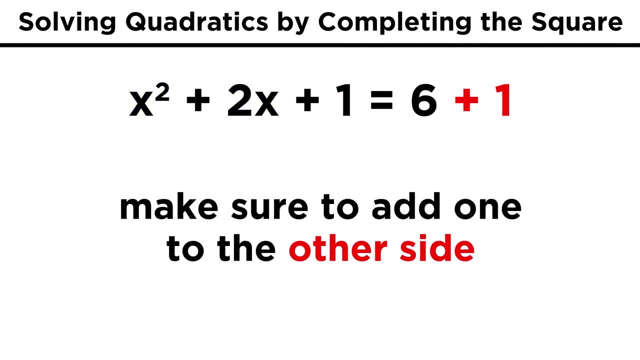 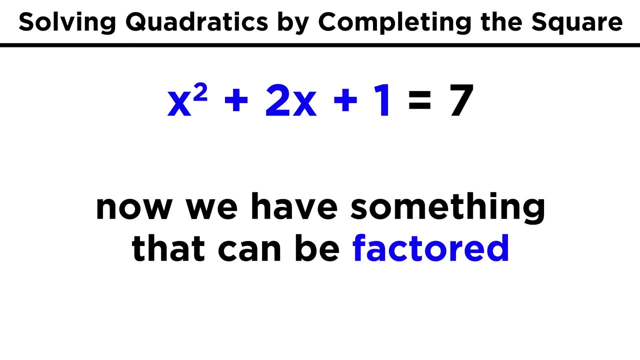 add one, so that we suddenly do have a perfect square polynomial, in essence completing the square. Well, whatever we do, we have to do it to both sides, so we end up with x squared plus two. x plus one equals seven. The reason this is useful is that we can now express the left side as x plus one quantity. 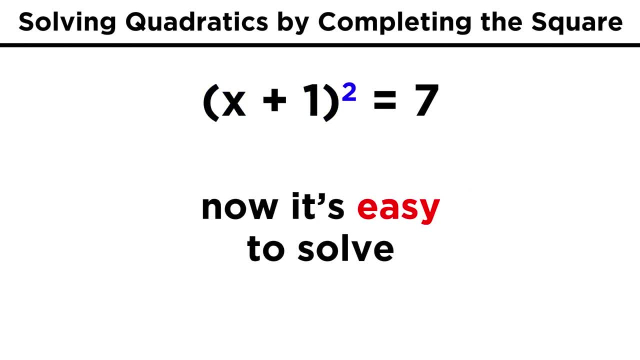 squared. From here it's not very hard to solve. We have an exponent of two, so we take the square root of both sides. That gives us x plus one equals plus or minus root seven. Remember that when taking the square root of the square root of both sides, we take 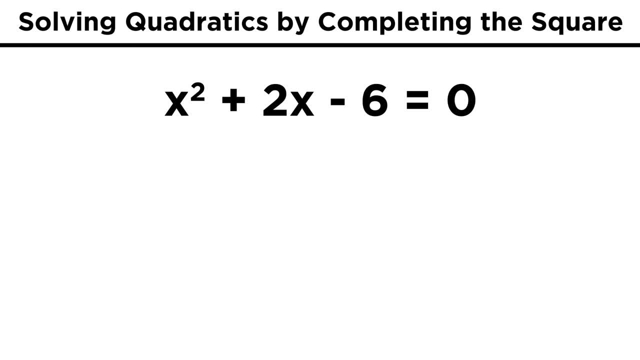 Let's say we have x squared plus two. x minus six equals zero. If we find the factors of negative six, which are combinations of one and six or two and two and three, we find that there is no way to add any pair of factors together to get. 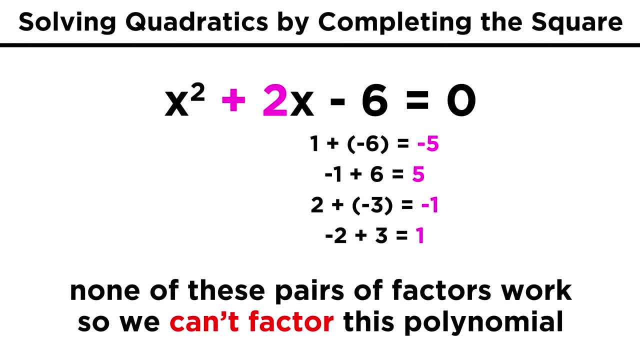 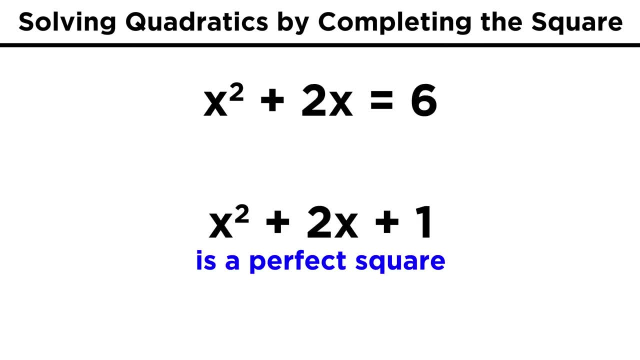 positive two. so we can't factor this polynomial. But let's do a little trick. Let's add six to both sides, bringing the six to the other side. Earlier we saw that x squared plus two, x plus one is a perfect square. so what if we now 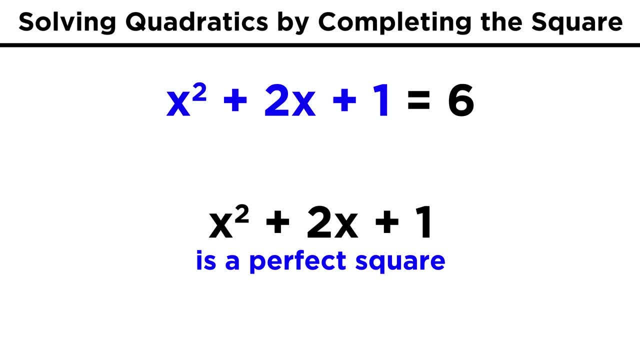 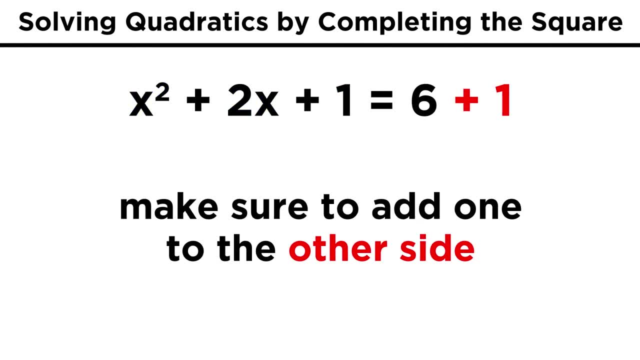 add one so that we suddenly do have a perfect square, polynomial, in essence completing the square. Well, whatever we do, we have to do it to both sides, so we end up with x squared plus two. x plus one equals seven. 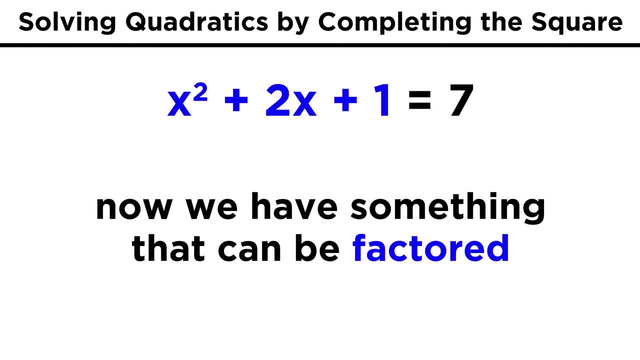 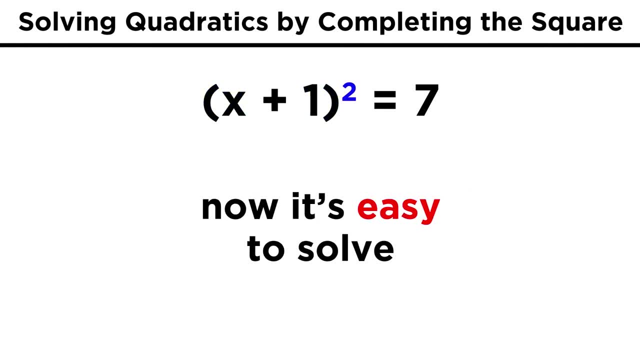 The reason this is useful is that we can now express the left side as x plus one quantity squared. From here it's not very hard to solve. We have an exponent of two, so we take the square root of both sides. That gives us x plus one equals plus or minus root seven. Remember that when taking the square root of both sides, we have an exponent of two, so we take the square root of both sides. Remember that when taking the square root of both sides, we have an exponent of two, so we take the square root of both sides. 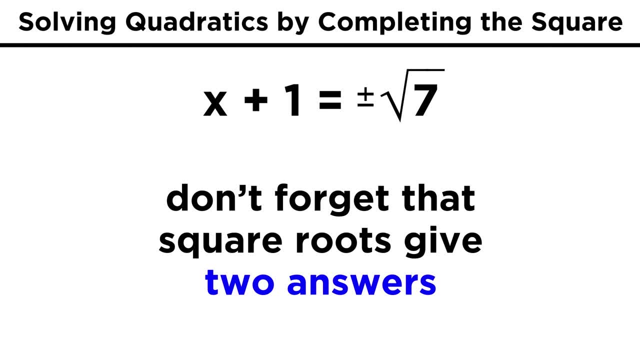 And when, taking the square root of both sides, we have an exponent of two, so we take the square root of both sides. Well, now, with the square root of a number, we get two answers, since both of these square to give seven. 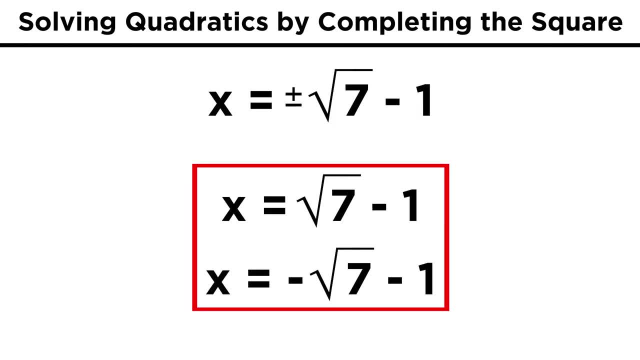 Now we subtract one to solve for x, and the right side can now be expressed as two values: either root seven minus one or negative root seven minus one. While these are not as aesthetically pleasing as integers, they are indeed the two solutions. 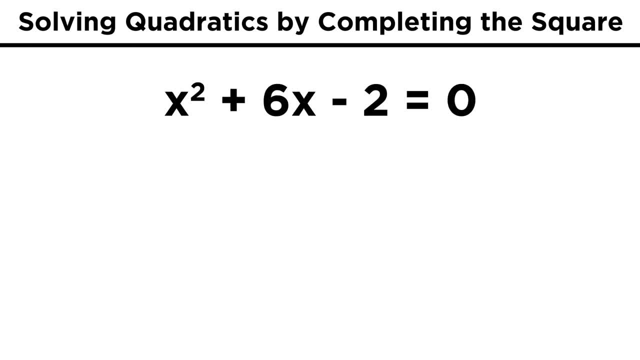 to this polynomial. Let's try another. say: we have x squared plus six. x minus two equals zero, equals zero. Once again, we would quickly see that this can't be factored. so let's bring two to the other side. Now to complete the square, all we do is take this coefficient of X, in this case six, and 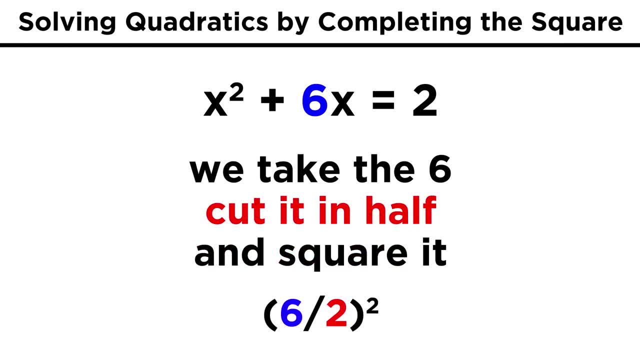 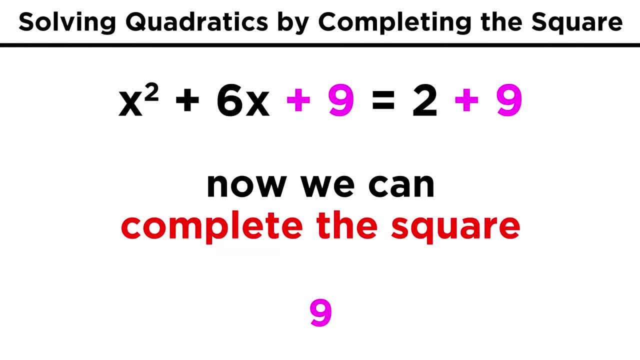 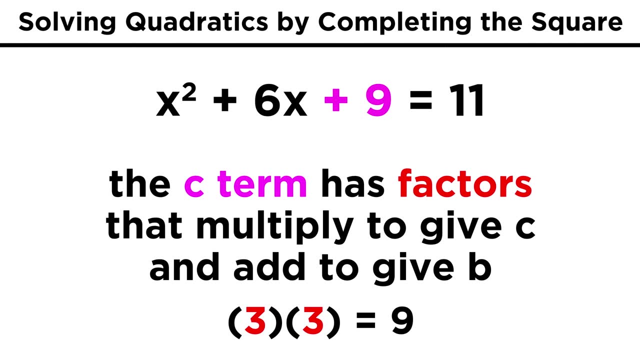 we must cut it in half and then square it. Six divided by two is three, and then we square that to get nine. We add nine to both sides to complete the square, leaving us with this expression. The reason we do this is because we need a C term with factors that multiply to give. 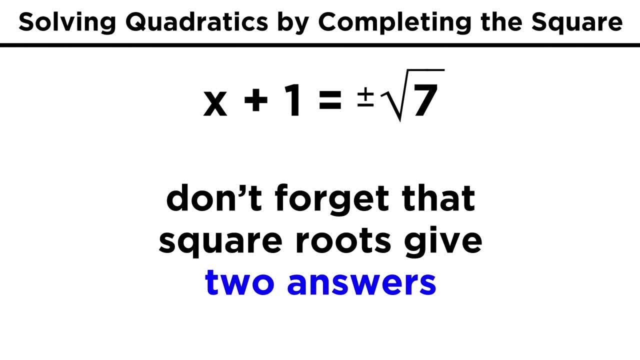 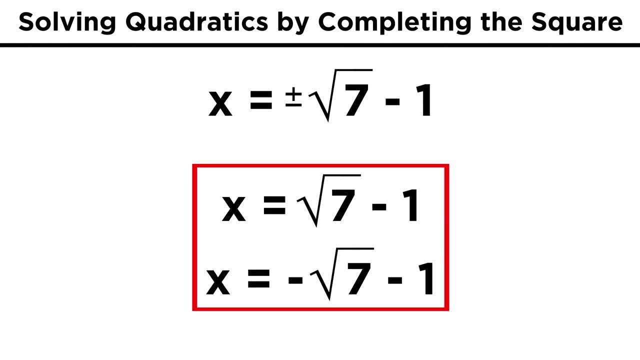 square root of a number, we get two answers, since both of these square to give seven. Now we subtract one to solve for X, and the right side can now be expressed as two values, either root seven minus one, or negative root seven minus one. 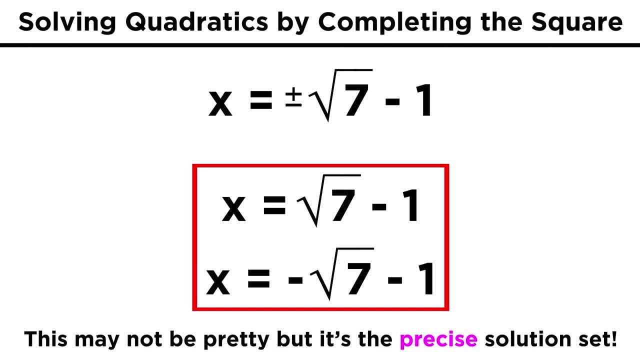 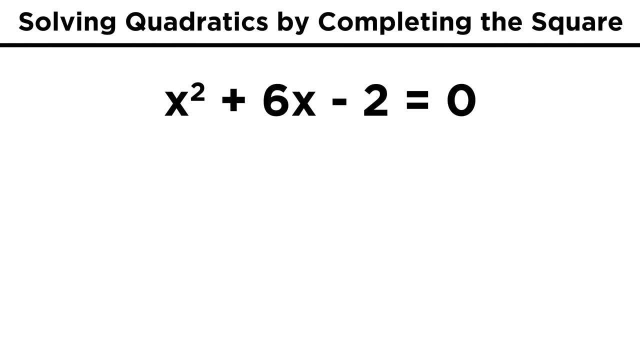 While these are not as aesthetically pleasing as integers, they are indeed the two solutions to this polynomial. Let's try another. say we have X squared plus six. X minus two equals zero. Once again, we would quickly see that this can't be factored, so let's bring two. 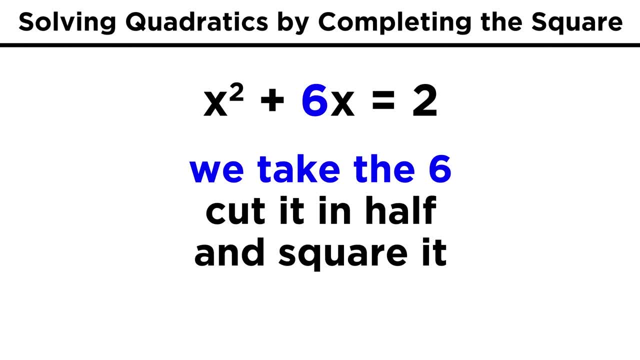 to the other side. Now, to complete the square, all we do is take this coefficient of X, in this case six, and we must cut it in half and then square it. Six divided by two is three, and then we square that to get nine. 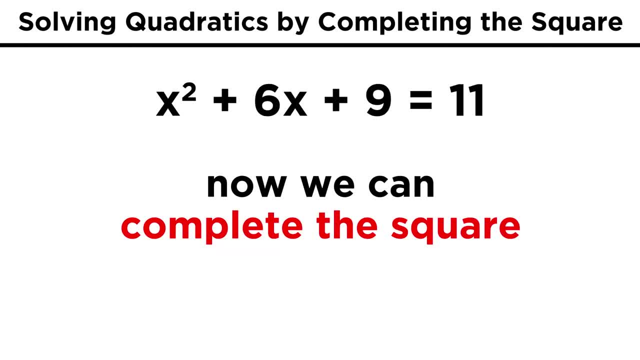 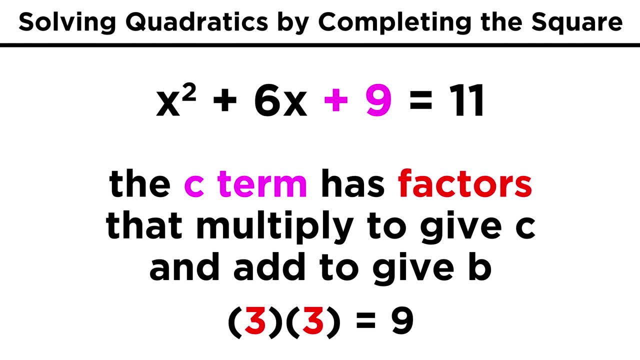 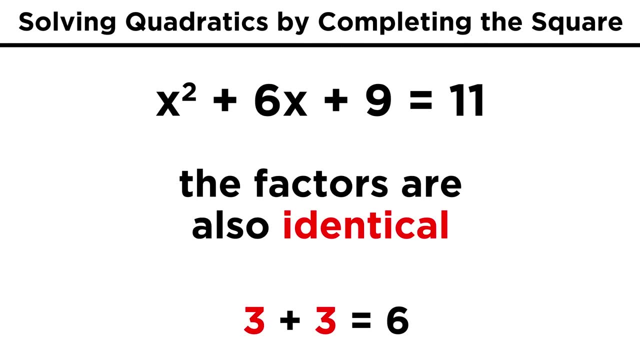 We add nine to both sides to complete the square, leaving us with this. The reason we do this is because we need a C term, with factors that multiply to give C and add to give B. But since it's a perfect square, the factors must be identical. so 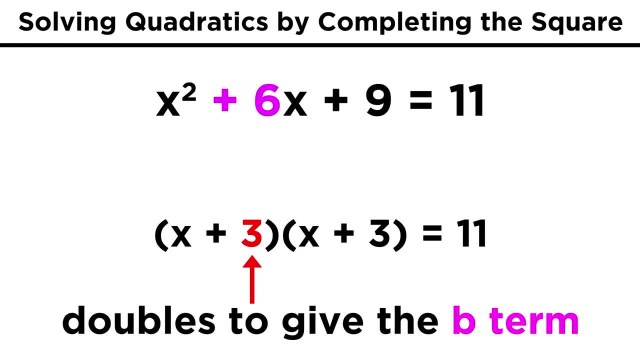 that factor must be the square root of C and at the same time add to itself or double to give B. So when doing these problems, just cut the X coefficient in half to get the factor that will go in the binomial. 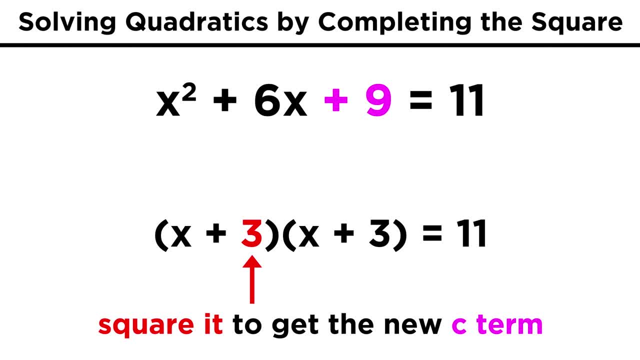 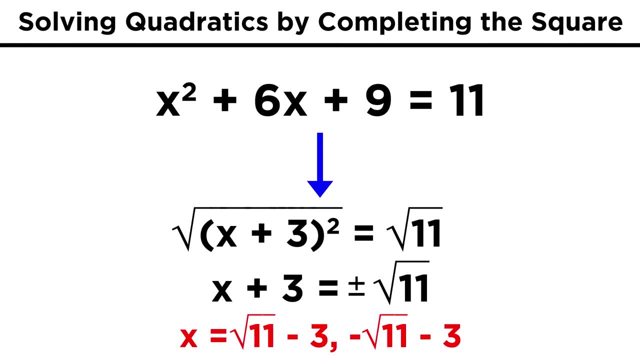 And then square it. to get the C term, you must add to both sides, and that's all you need to worry about Now. we do have a perfect square. so we get X plus three. quantity squared equals eleven. Take the square root and subtract three and we get X equals root, eleven minus three, or 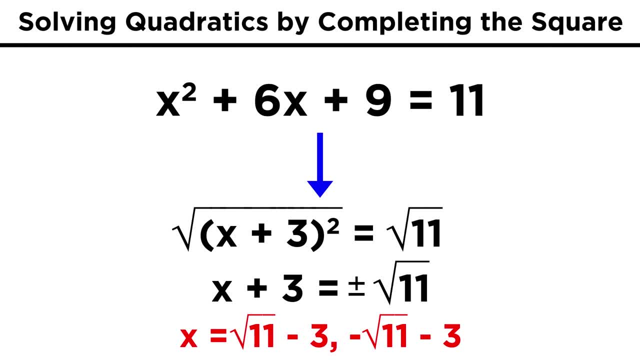 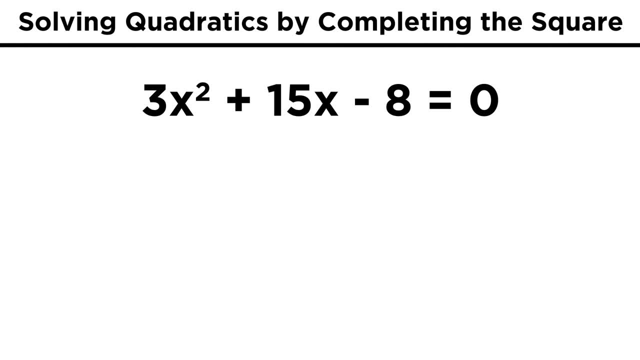 negative root: eleven minus three. Let's do just one more. Three X squared plus fifteen, X minus eight equals zero. Let's do just one more: Three X squared plus fifteen, X minus eight equals zero. Once again we bring eight to the other side. but now we have something trickier on the 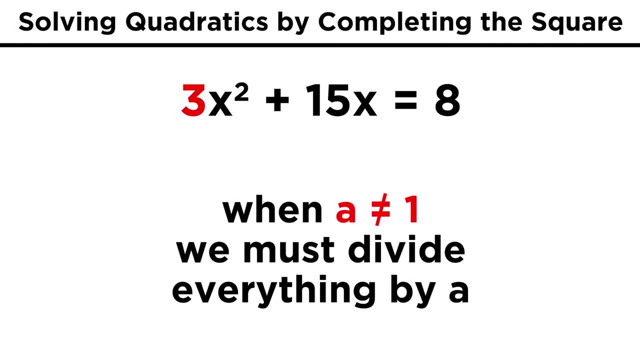 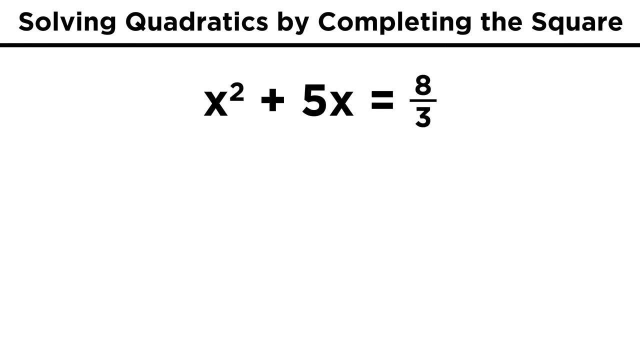 left. The best thing to do when there is a coefficient on the x squared term is to divide everything by that coefficient. You may end up with fractions, but this is definitely the easiest way to go, even if that's the case. So let's divide everything by three. 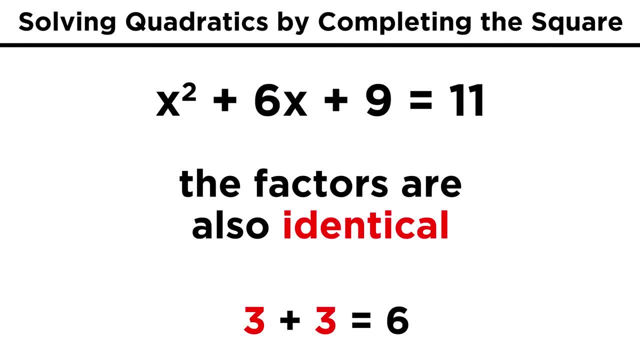 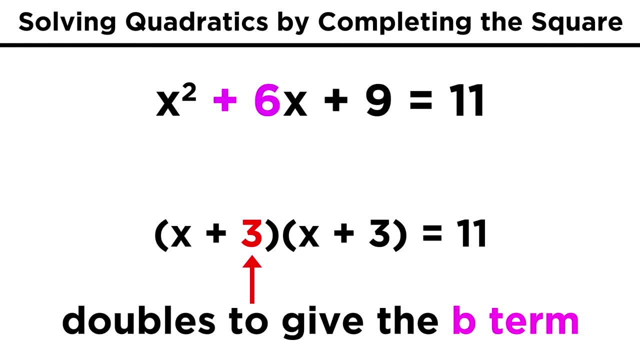 C and add to give B. But since it's a perfect square, the factors must be identical, so that factor must be the square root of C and at the same time add to itself or double to give B. So when doing these problems, just cut the X coefficient in half to get the factor. 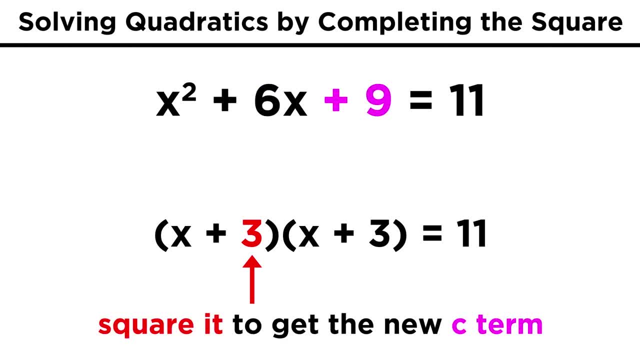 that will go in the binomial and then square it. to get the C term, you must add to both sides And that's all you need to worry about Now. we do have a perfect square, so we get X plus three. quantity squared equals eleven. 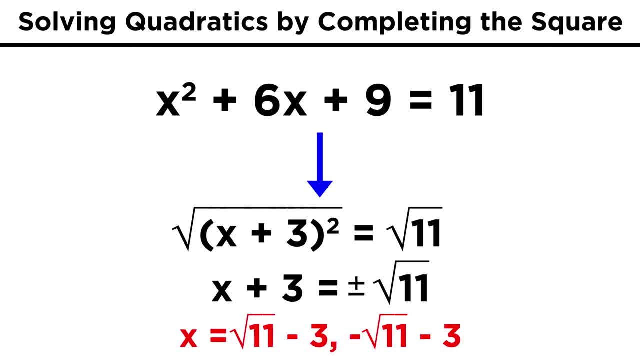 Take the square root and subtract three and we get X equals root eleven minus three, or negative root, eleven minus three. Let's do just one more: three X squared plus fifteen. X minus eight equals zero. Once again, we bring eight to the other side. 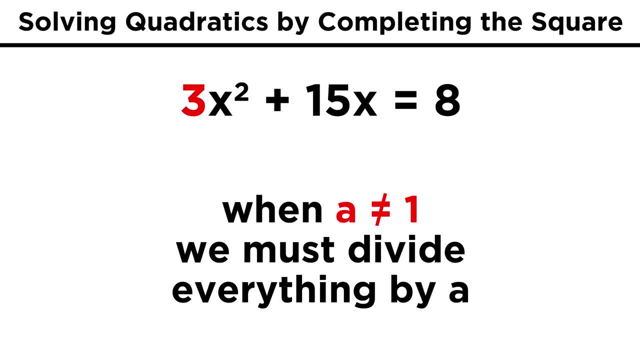 But now we have something trickier on the left. The best thing to do when there is a coefficient on the X squared term is to divide everything by that coefficient. You may end up with fractions, but this is definitely the easiest way to go, even if 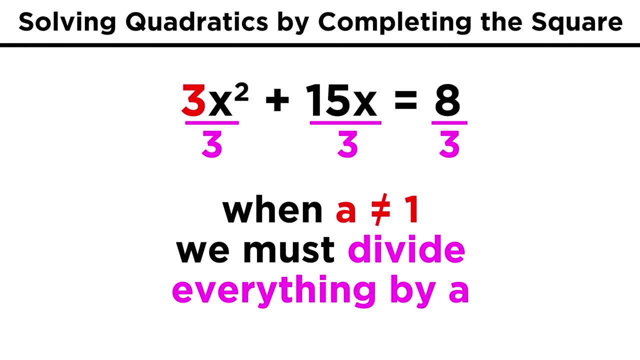 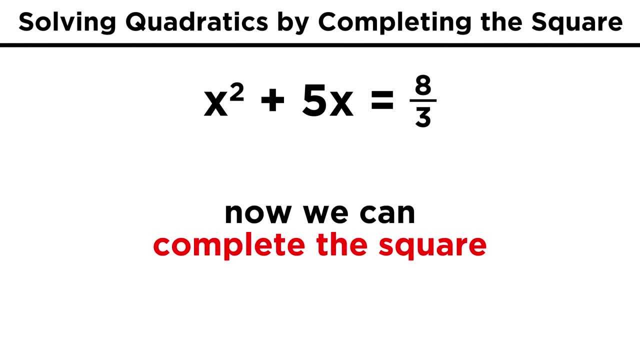 that's the case. So let's divide everything by three. We will get X squared plus five X equals eight thirds. Now we can complete the square With five. it may seem messy, because cutting in half gives five X's, So let's do that. 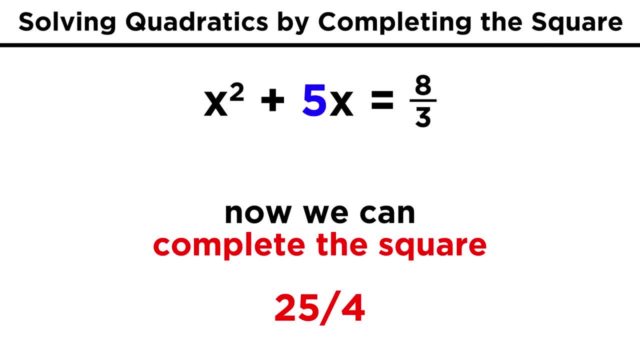 We get five halves, which then squares to give twenty-five fourths. But if that's what we get, then that's what we have to work with. We add that to the right side as well. find the least common denominator, which is twelve. 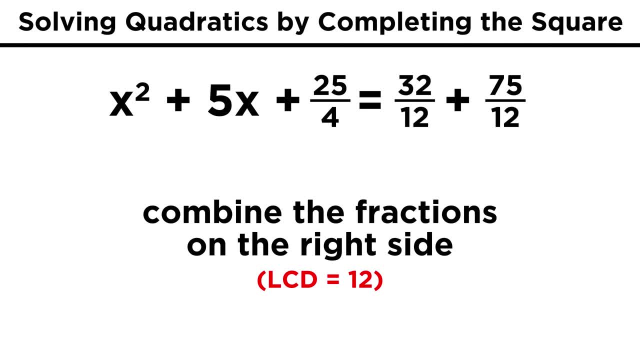 and convert these fractions to thirty-two twelfths and seventy-five twelfths so that we can add them together to get a hundred and seven twelfths. Now we factor the left side to get X plus five- halves quantity squared. So that's what we have to work with. 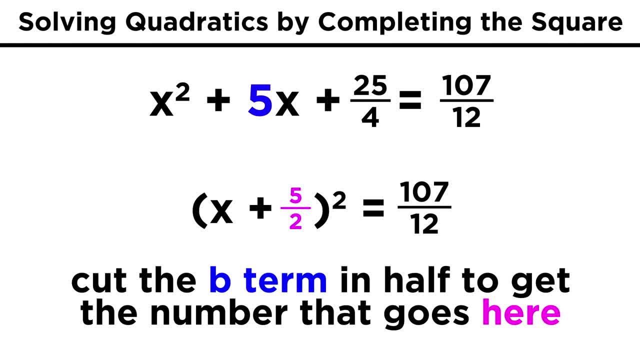 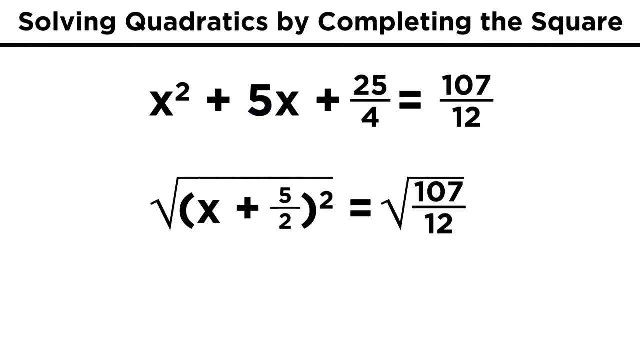 Remember, when we cut that initial B term in half before we square it, that's the number that will end up in the resulting binomial. Then, just like the other examples, we take the square root of both sides and subtract five halves, which will allow us to express the two solutions for X. being sure to simplify,